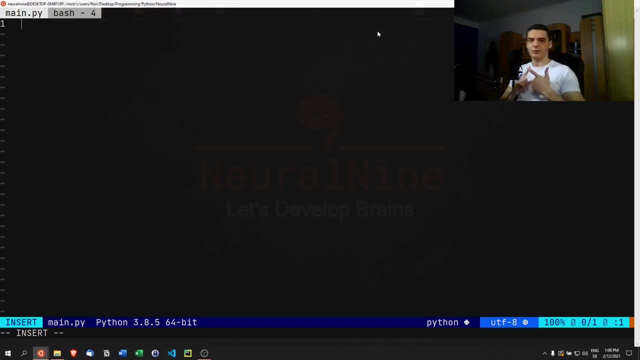 if you want to use them in larger projects. So you don't want to use them in your 50 line python script, You want to use them in big applications. we have multiple classes and multiple python files and modules working together, Because otherwise they're just increasing. This is 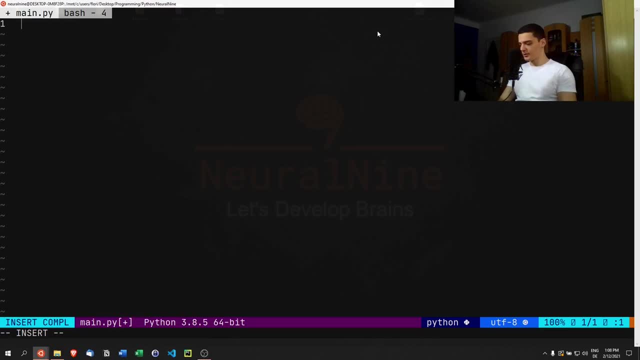 just looking at an example here. let's say we have an abstract class person. So for this we need to say: from ABC, which stands for abstract class, import, ABC meta and abstract abstract static method. there you go, And now we're going to create a person interface. So we're going to say: 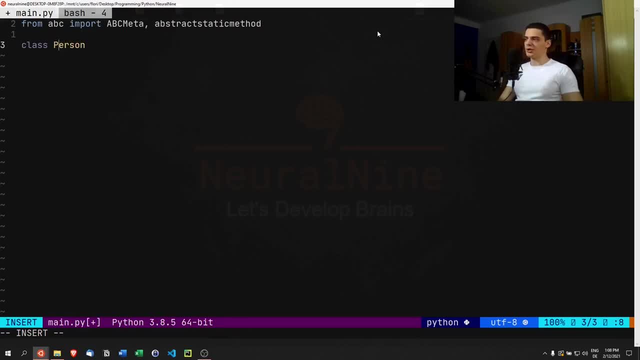 class person. And one notation that is best practice or the convention is: if something is an interface, because in Python we cannot just say interface person. if something is an interface, we call it I whatever, So I person in this case. and here we're going to say: meta equals ABC, meta. 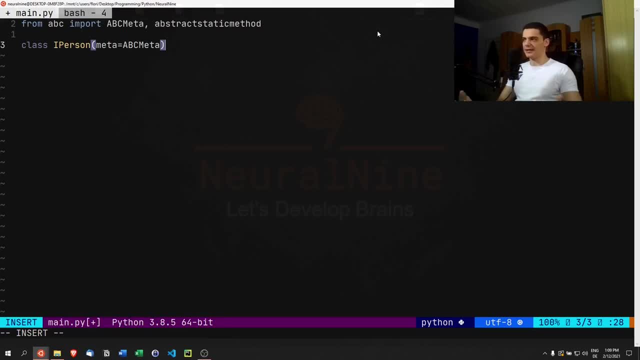 which basically means that this is an abstract class. we cannot create any instances of it. we're going to see what that means in a second. And then we're going to say abstract static method And we can say, for example, def person method. this is just a basic method that every person 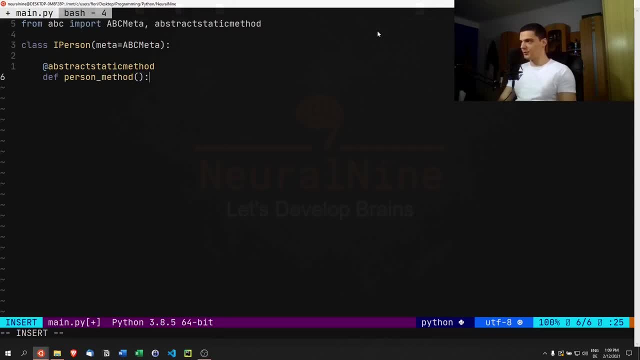 has. And then we're going to say, for example, this is just a basic function, And here we're just going to add a comment that this is an interface method, because the interface, the what an interface basically is, is just a definition of the signature. So we know, okay, we're going to have 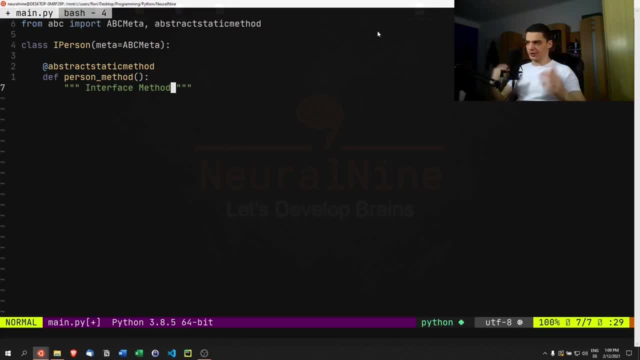 those functions, those methods, but we're not going to say what they actually do. So this is just mentioning that each person has to implement the person method. So we're going to see that this doesn't work, Because if I now say p one equals I person, for example, like that, and then 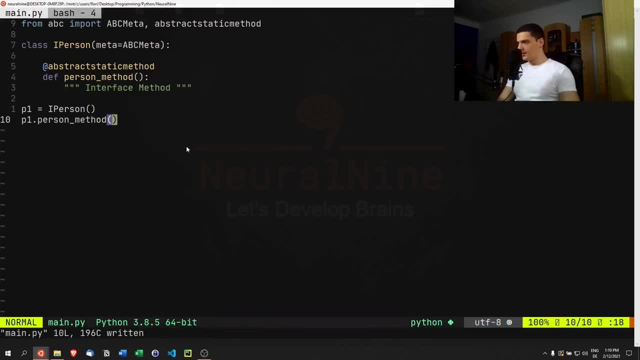 p one dot person method or something. Now I write this: we're going to see that this is not possible Because it's an abstract class. we cannot just go ahead. and actually one thing I made a mistake here: meta class is ABC meta. 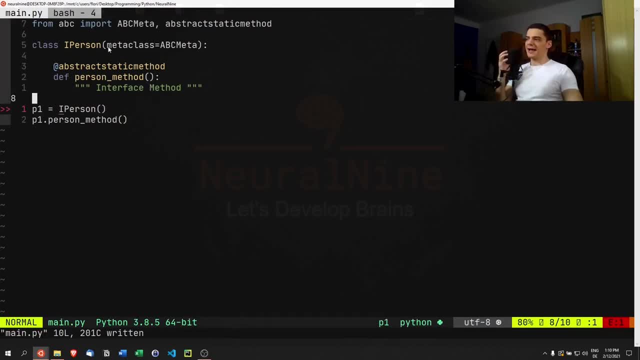 Then it's not going to work. This basically means that we're creating abstract class, And the definition of an abstract class is that we cannot create instances of it. So you're going to see here that we get the error abstract class. I person With abstract methods. we cannot instantiate this And we're going to see the 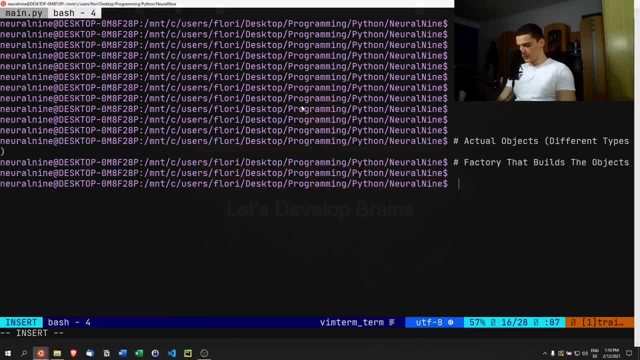 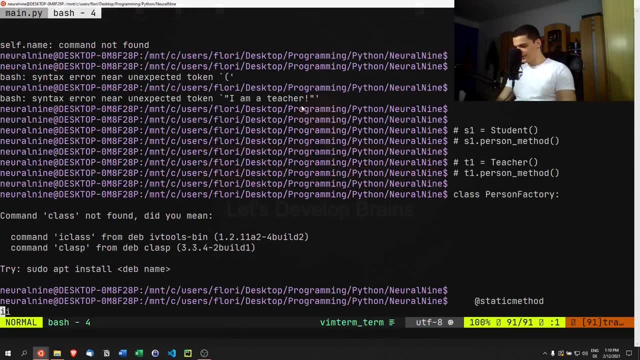 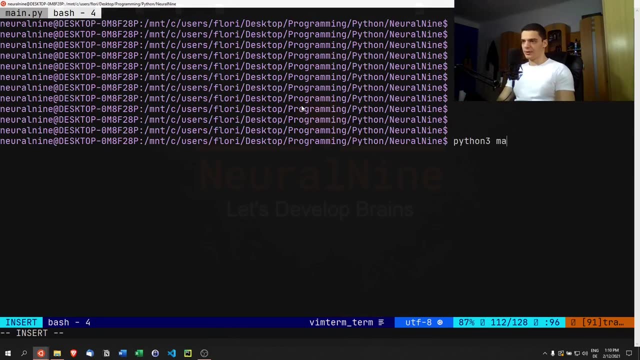 terminal. If I now go ahead and run Python, oh shit, what's happening here? Okay, I use the paste here. Let me just clear this real quick. They go Python three main dot py. You can see I can't instantiate the. 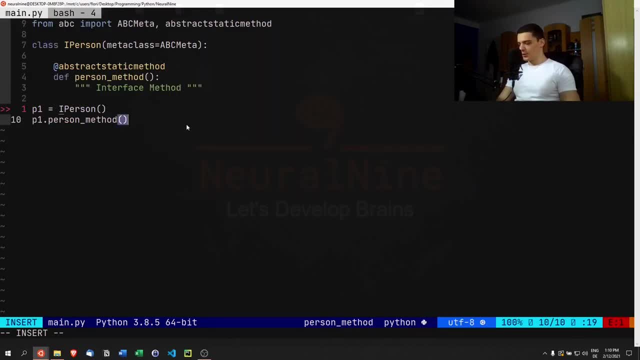 abstract class I person. So that's exactly what we want, actually. And now we're going to have another class student which is going to to inherit from this I person interface, is going to implement that I person interface And we're going to override this method. Now, if I don't do that, if I just say I 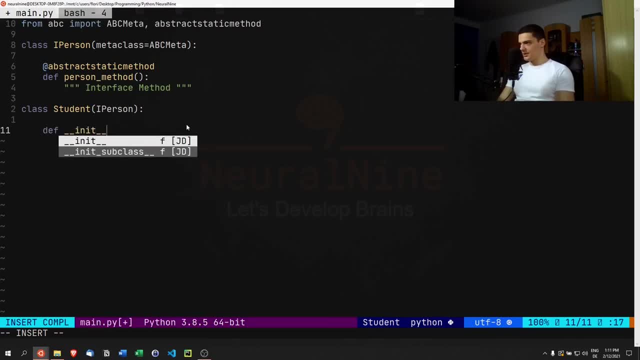 don't know if in it and I have a basic constructor here with I don't know self dot name equals basic student name. it's a default name. Then if I try to say s one equals student And we're actually just that we're not going to. 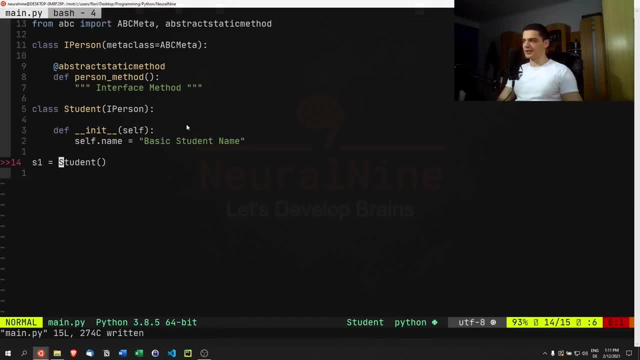 be able to create an instance of student, because student did not override the abstract static method, person method. we need to do that, Otherwise we cannot treat this as an instance of student. So we're going to do this as a non abstract class. So after the constructor we're going to say deaf person method with a self keyword. 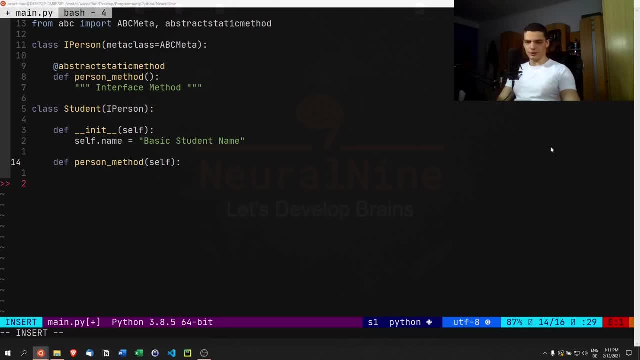 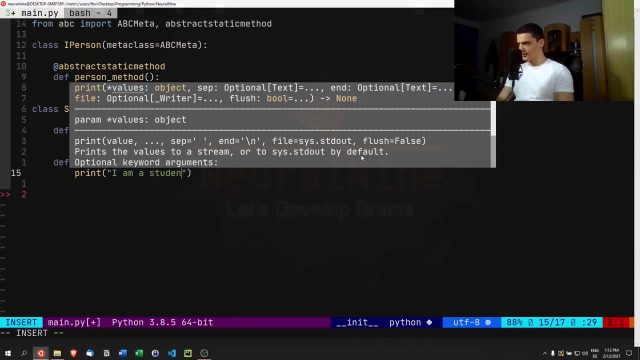 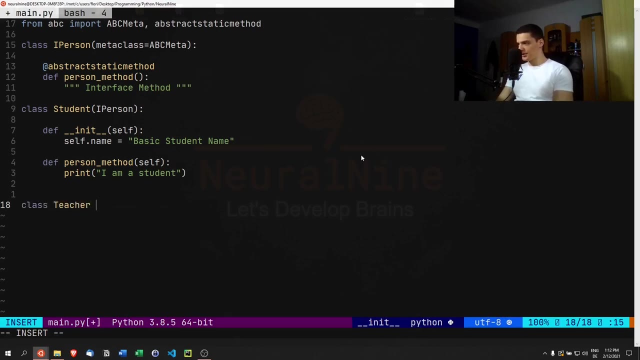 here. Actually, do we need to self keyword? Yeah, I mean, we don't need it. I'm not sure if we need it, But we're going to just say print: I am a student, like that. So this is the basic student class, which is also a person, And then we're going to have another one which is a teacher. 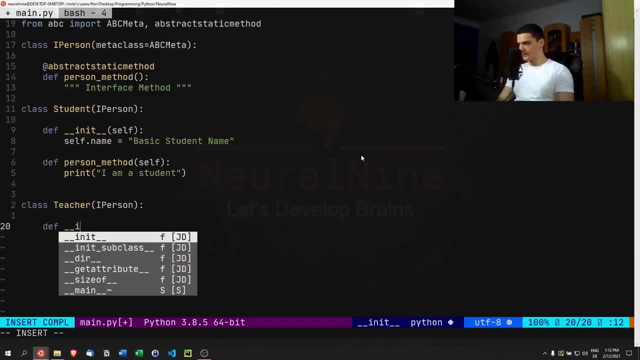 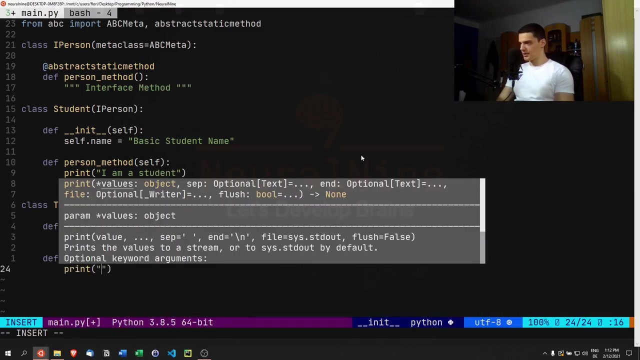 And there's also going to be a person And we're going to also have an init method, So a constructor, basically self dot name equals basic teacher name, And then we have person method Self again, And now we say print: I am a teacher. this is basically just for us to see if the object is a teacher or a student. 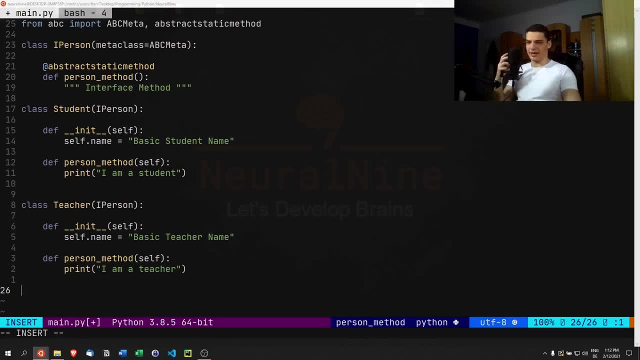 And now what we can do here, of course, is in Python. we can just go ahead and create those objects by seeing as one equals student, student, and then I can say: as one person method, And here I can say: t one equals teacher. 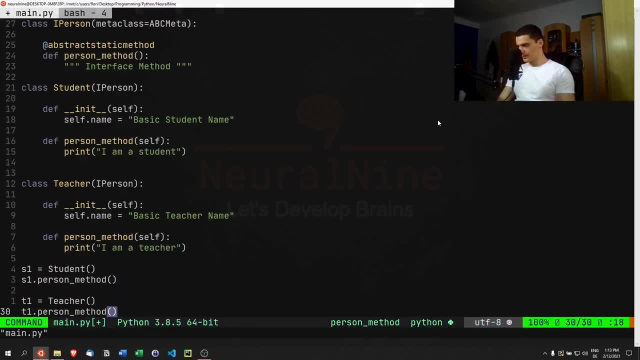 T one Dot person method. So we can now go into the terminal here and run this again. You can see, I'm a student, I'm a teacher. So that's a very basic style of learning. So that's a very basic stuff. What we now want to have is we want to decide during runtime. 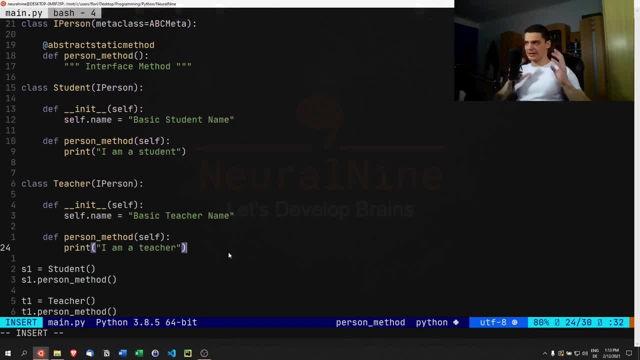 we know that we want to create a person method, a person class, sorry, a person object, But we don't know if this object shall be a student or a teacher, And we want to decide that dynamically during runtime. So one way to do that- this is the the not so beautiful way to do it- is to just say: 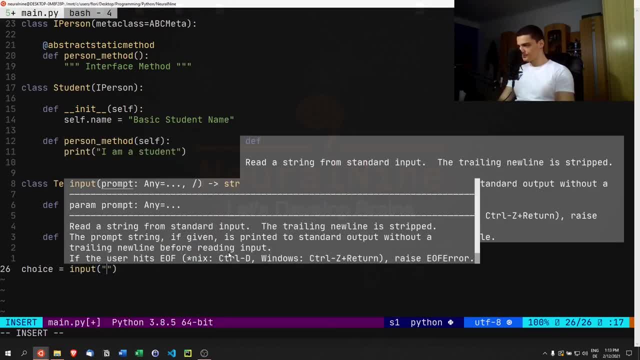 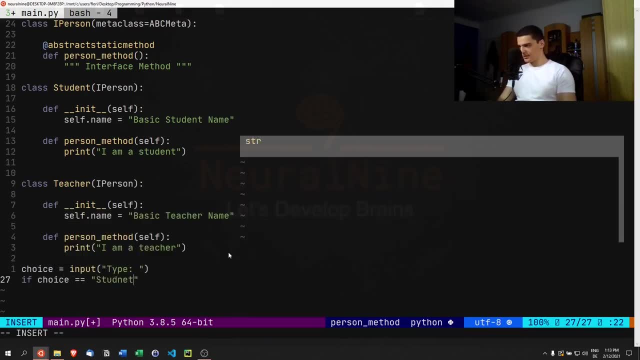 I don't know. choice equals input type or something, And then we can just say, okay, if the choice is student, then just go ahead and create a student and so on. But that's not the factory design pattern. The factory design pattern is to now have a factory class, which 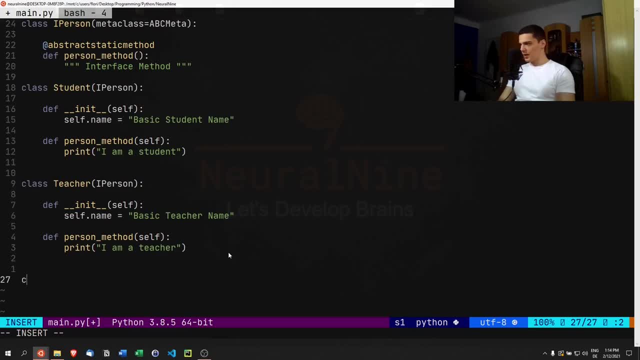 actually builds person objects. So we actually want to say class person factory And this person factory is going to build the person that we want to build. So we're going to say def, build person or get person or produce person, call it whatever you want, I'm not sure. 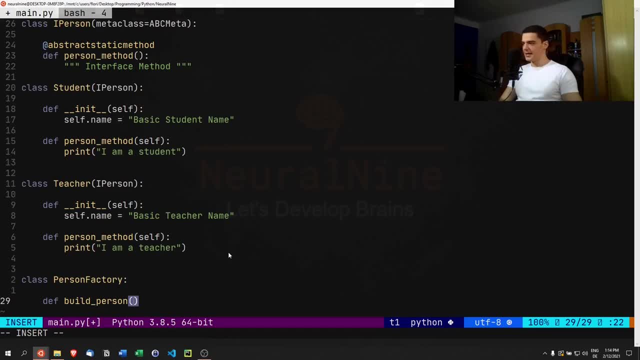 what the best practice definition or the best practice name here is, And what we're going to pass here is the type. So we're going to pass the type of the person by saying person type And this is, in our case, just going to be a string. 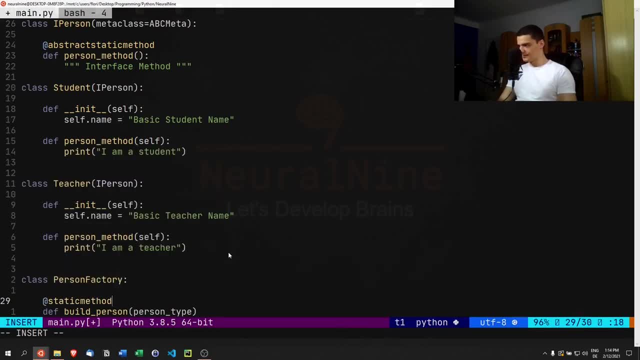 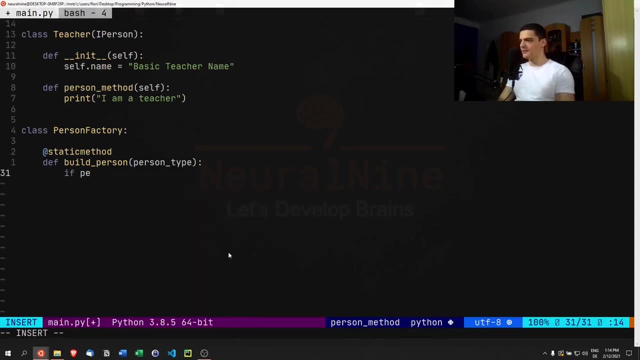 And, by the way, this, of course, is a static method. So we're going to say: build person And what we're going to do here is we're just going to say, okay, if the person type is student, then we're going to return a new student. 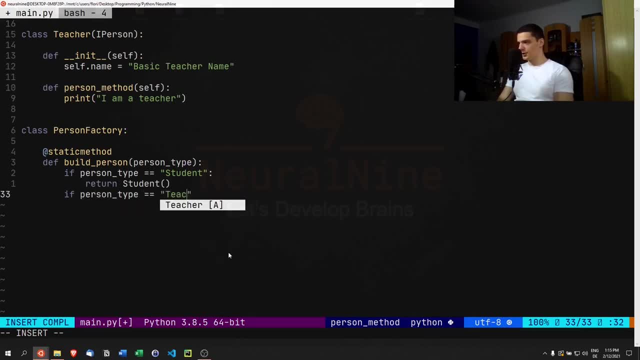 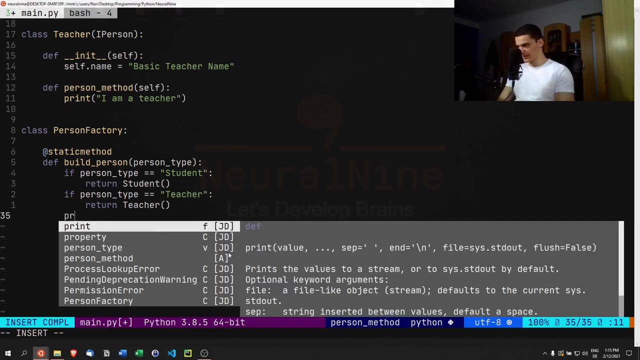 Then if the person type is teacher, we're going to return a new teacher object And what we're automatically doing here is going to be a system. So we're going to open this up And let's say it's a class type And what it's going to do is you're going to move it to their 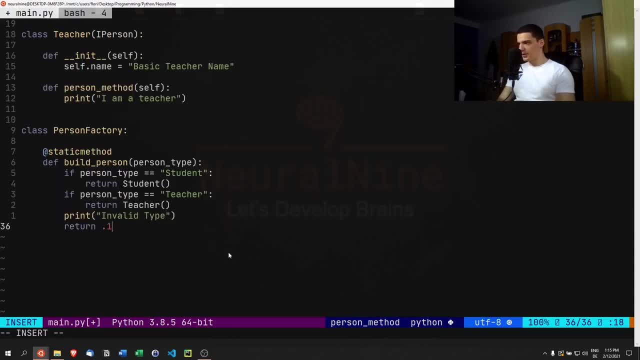 page. And then what happens when the package goes to class type? Well now I'll just say etiquette as well, So you can go back to class type and there it is. If the page is somebody who asks for free, clearly I would click on the accept button there. So let's take a look. So one of the things 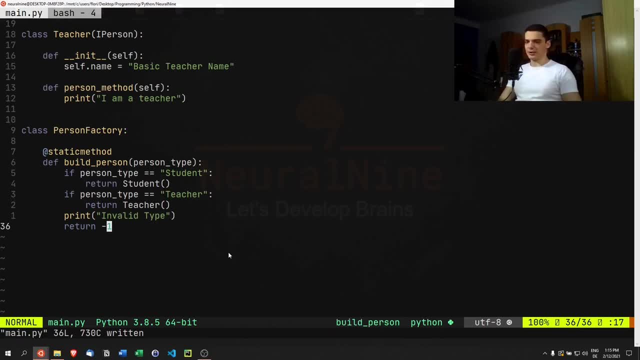 that happened in here is a list of fields. Okay, okay, All right, Yeah, Yeah, okay Yeah. And now what we can do is we can actually go ahead and create this main section here And we can say that we can have the choice again. So we can say: choice input. 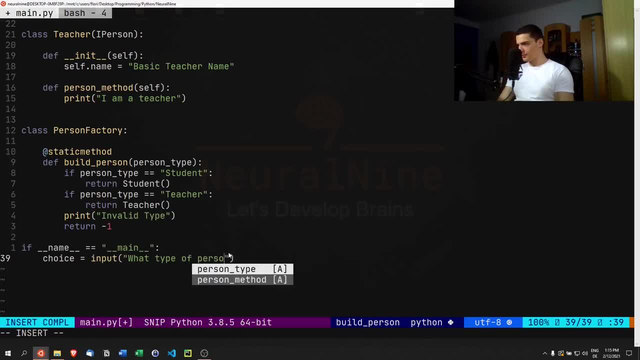 What type of person do you want to create? them backslash in here And then we can just create the person depending on that input. So we can actually go ahead and say person, sorry person, factory, dot, build person, depending on the choice. 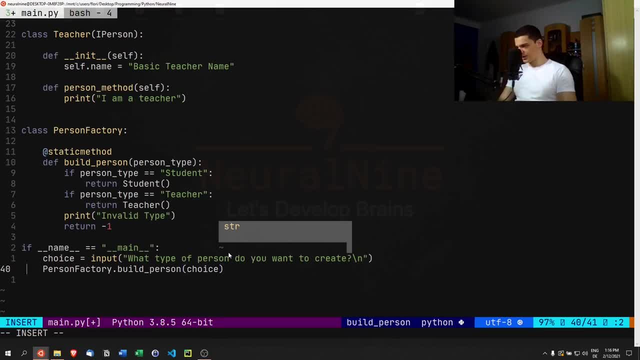 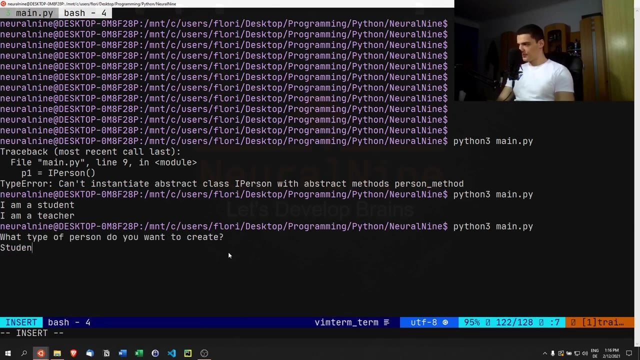 And then once we have that person, actually we need to save it in an object here, So we need to say person equals that and then we can say person dot, person method. And you're going to see that if we now run this, I can enter student, for example. 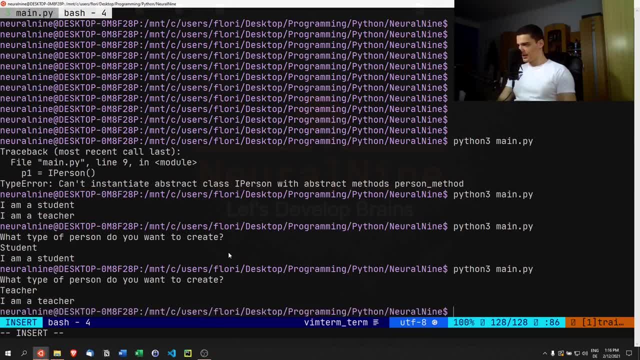 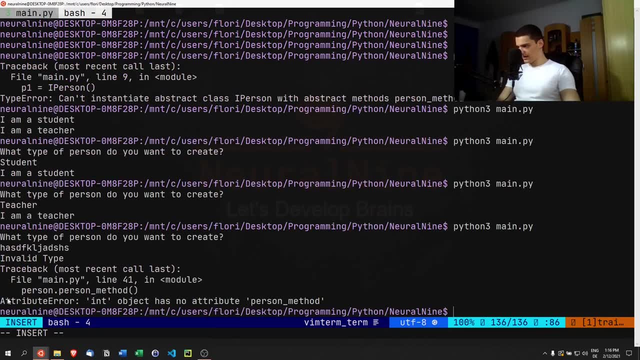 and I'm going to get. I'm a student, I can enter teacher and get them getting. I'm a teacher and I can enter something else and we're going to get invalid type and an attribute error and so on. But, as you can see, we can dynamically decide if we want to build a student. 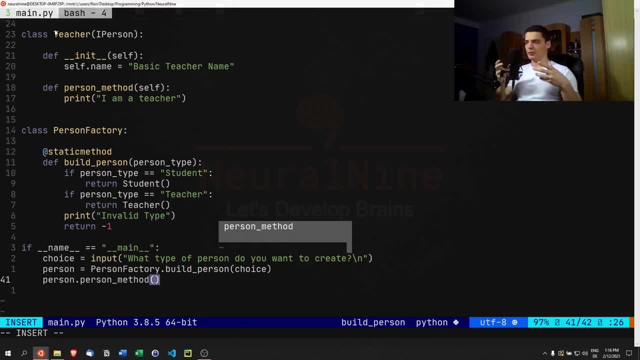 or a teacher during runtime. So we don't have to know in advance, we can do it on the fly in the practical. So if we wanted to build a student or a teacher during runtime, we could just set. a Factory. pattern is very useful if we want to do this quite often, because then we can just reuse this factory. 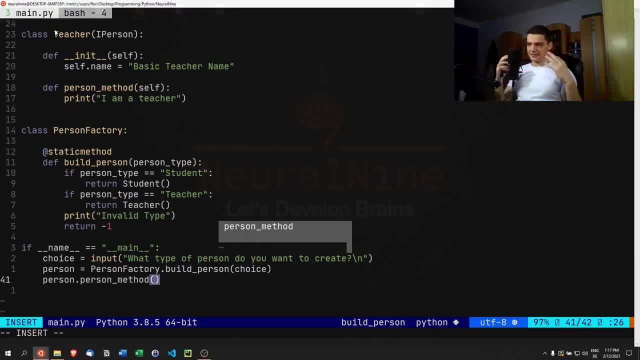 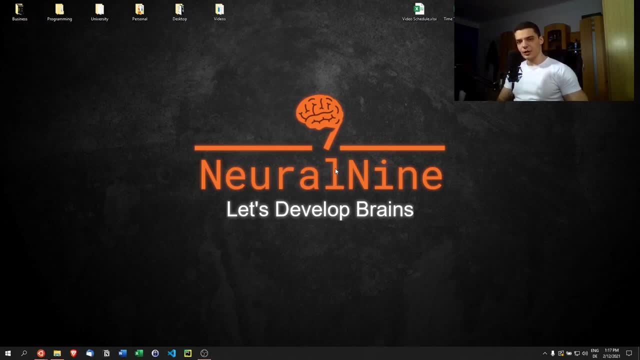 We can just say factory, build person and then pass the type. So that's it for this video. Hope you enjoyed and hope you learned something. if so, Let me know by hitting a like button and leaving a comment in the comment section down below. and, of course, don't forget to subscribe.